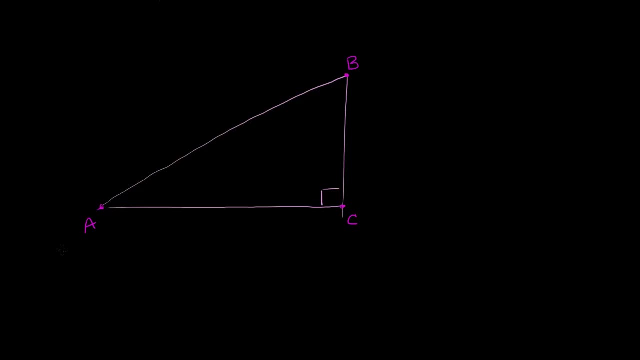 What I want to do in this video is prove that the circumcenter of a right triangle is actually the midpoint of the hypotenuse, And to do that, I'm going to first take a look at the perpendicular bisector of one of the legs of this right triangle. 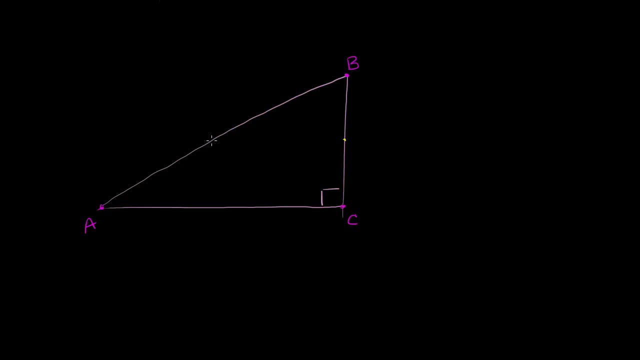 So let me construct the perpendicular bisector of leg BC right over here. So it's going to look something like this: It intersects at a right angle, It's perpendicular and it bisects it. So the distance from B to this point, which we'll call M, 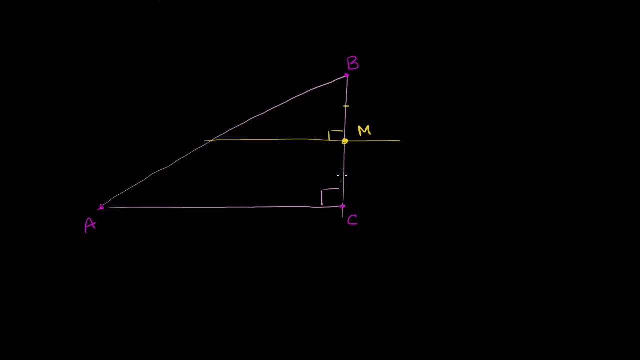 maybe M for midpoint is the same as the distance from M to C. So those two distances are going to be equal And let's call the point where this perpendicular bisector intersects the hypotenuse. let's call this O, And we're going to prove that O is the circumcenter. 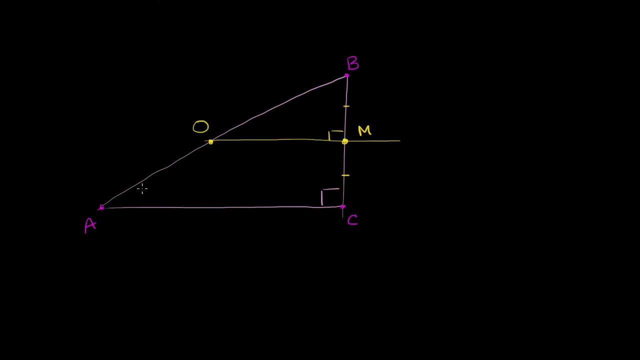 of this right triangle. Now, the first thing that you might realize- and this is what we've seen in many problems- the triangle OBM- OBM looks similar to triangle ABC And it's actually not too hard to prove. They both already have a 90-degree angle. 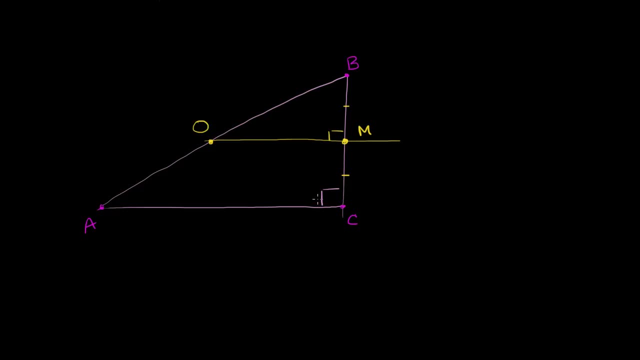 So if we show that they both have another set of corresponding angles that are congruent to each other, then we know that they're similar by AA similarity And they both clearly share this angle. right over here, OBC is part of the smaller triangle. 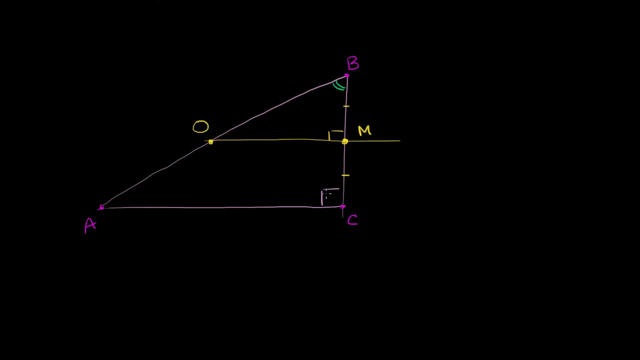 And ABC, which is really the same angle, is part of the larger triangle And they also obviously share a 90-degree angle. So by AA triangle similarity we have triangle OBM is similar to triangle ABC And what's useful about this is we 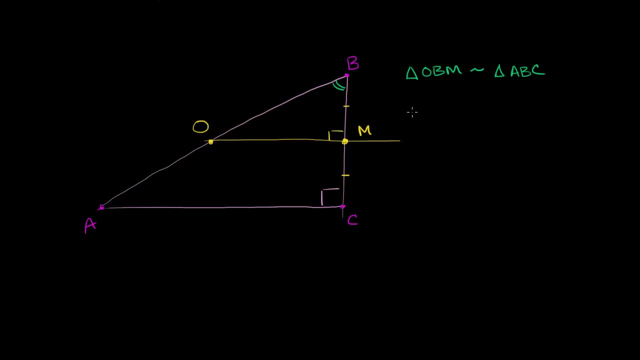 know that similar triangles, the ratios between corresponding sides are accosted. So, for example, we know that the ratio between side BM, which is on the smaller triangle, we know that the ratio between BM. let me do this in a different color. 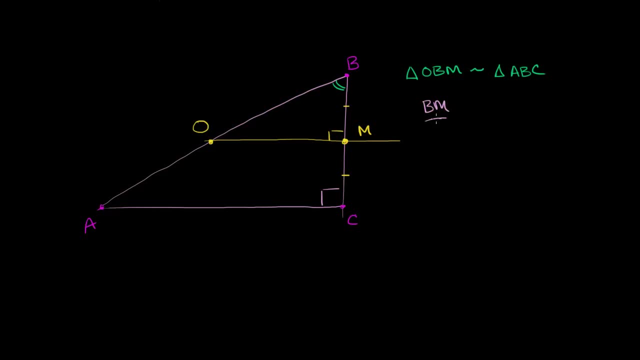 just for the sake of it. we know that the ratio between BM and BC, the ratio of this side on the smaller triangle to the corresponding side on the larger triangle, is going to be the same as the ratio of the hypotenuse on the smaller triangle, BO to the hypotenuse. 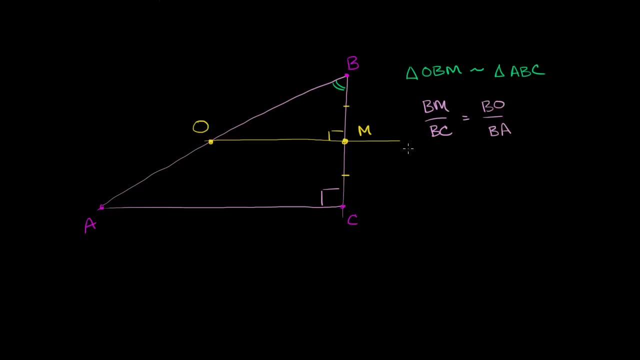 of the larger triangle because they are similar. Well, we know what the ratio of BM to BC is. BM is half of BC, So this ratio over here, the ratio of BM to BC, is going to be equal to 1 half. 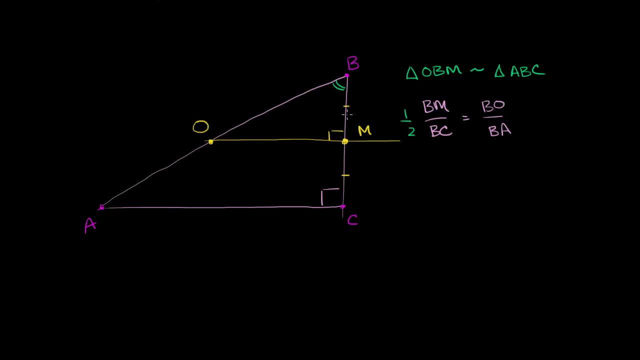 This is M, is the midpoint of these things. So this is exactly the same distance as this. So this is 1 half of the entire BC. So if 1 half is equal to BM over BC, is equal to BO over BA, we then know if we just kind of ignore this middle part, right. 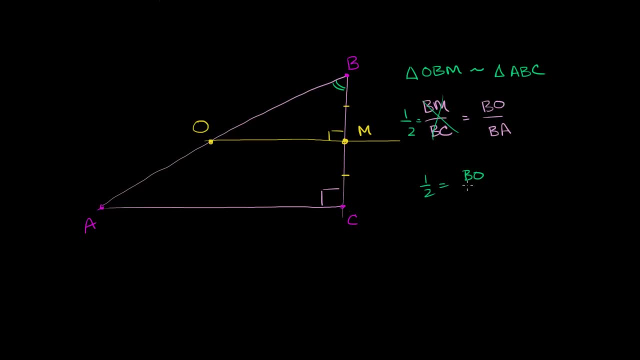 over here that 1 half is equal to BO over BA, And if you cross multiply it, we're going to see that. well, there's multiple ways to think about it, but you could just cross multiply and you'd say BA is equal to 2BO. 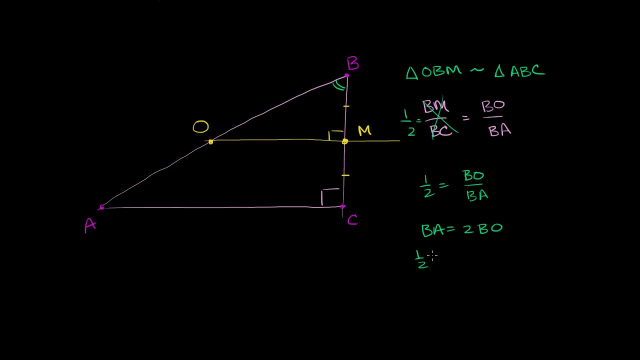 Or if you divide both sides by 2, and they're really equivalent statements: 1 half BA is equal to BO, So BO is 1 half of BA. So this is 1 half BA, And so this other length AO right over here. 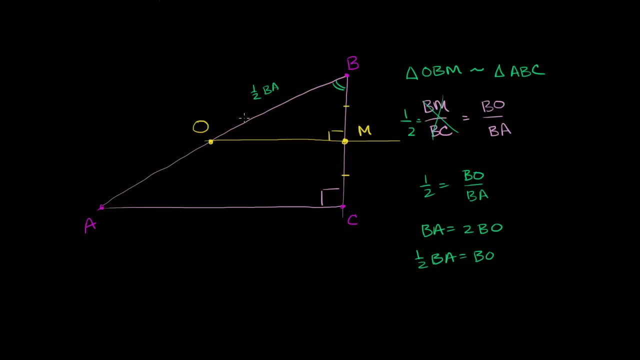 this is going to be BA minus 1 half BO Right, OK, 1 half BA. So this is also going to be 1 half BA, And so this segment right over here, AO is going to be congruent to OB. 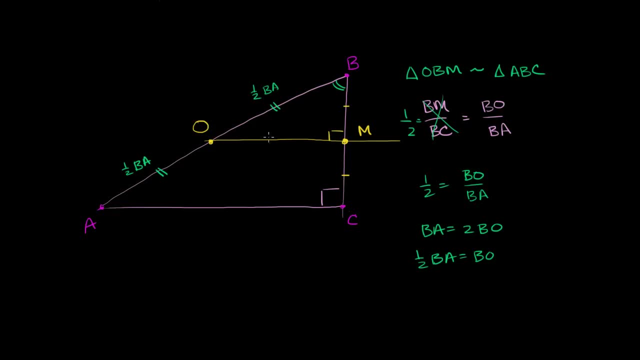 So what we've just shown, first of all, is that this perpendicular bisector right over here, the perpendicular bisector of segment BC, it intersects the hypotenuse of our right triangle at the midpoint. So we've already established, so one thing that we've already. 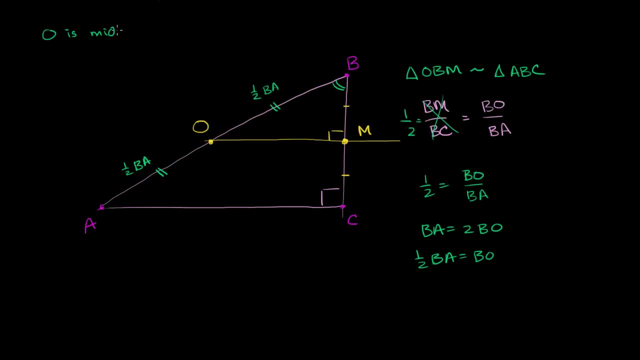 established is: O is the midpoint. OK, O is the midpoint of the hypotenuse AB. Well, that by itself is interesting. But we also know that if a point sits on a perpendicular bisector of a segment, it's equidistant from the endpoints of the segment. 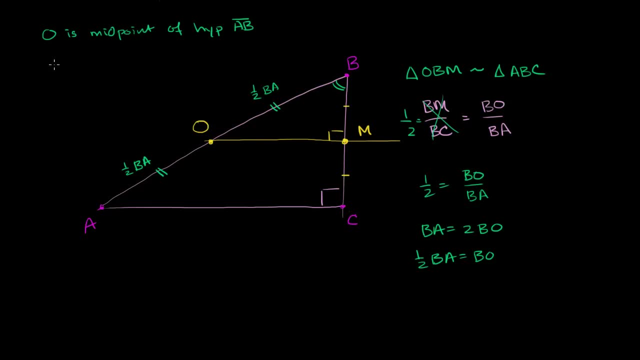 We showed that in a previous video. So we also know that OOB- it's equidistant from the endpoints of this segment right over here that OB is equal to AB. OK, OK, That should be equal to OC. But we know from this first statement right over here: